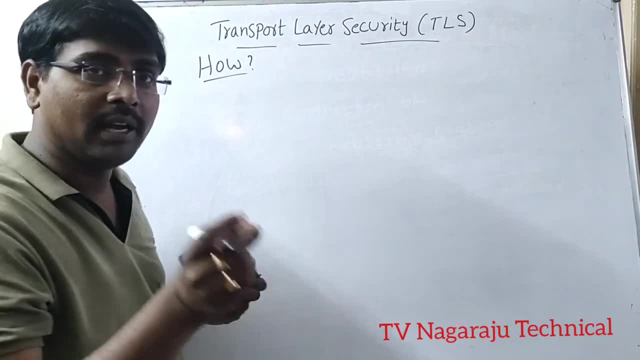 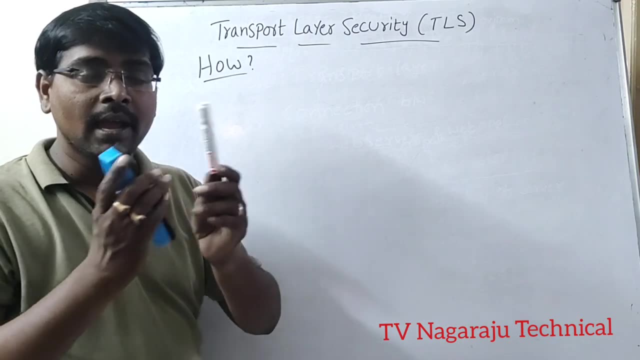 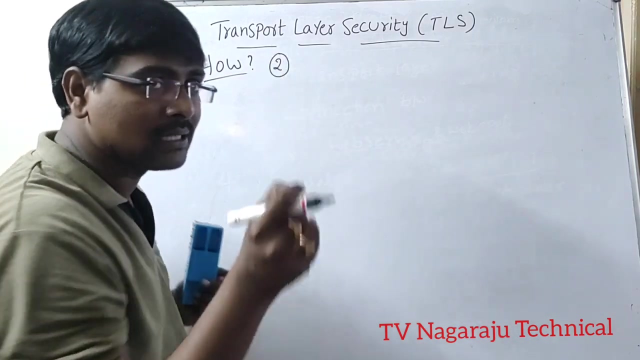 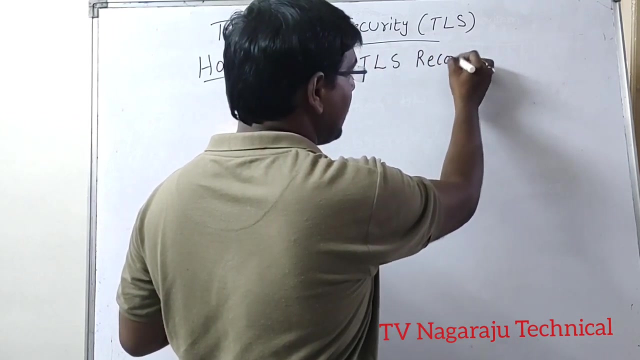 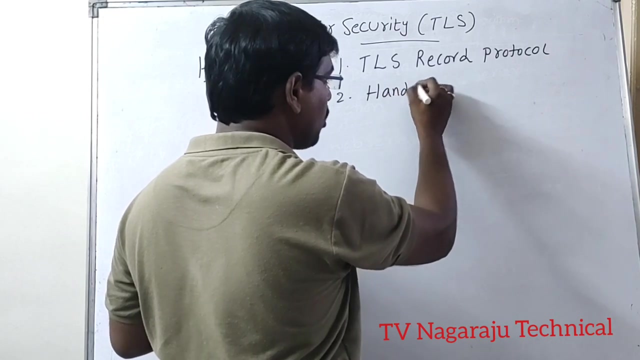 Simply transport layer. security uses both the symmetric and asymmetric encryption algorithms: Symmetric and asymmetric encryption algorithm. Mainly it depends on two layers. TLS mainly depends on two layers. The first one is TLS record protocol. The second one is handshake process. 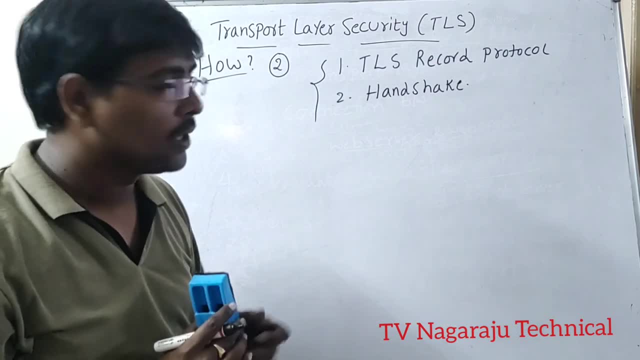 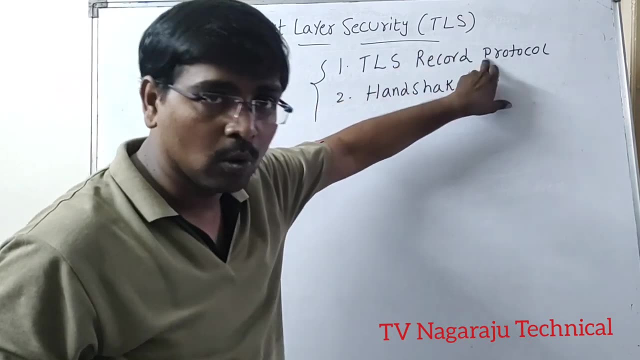 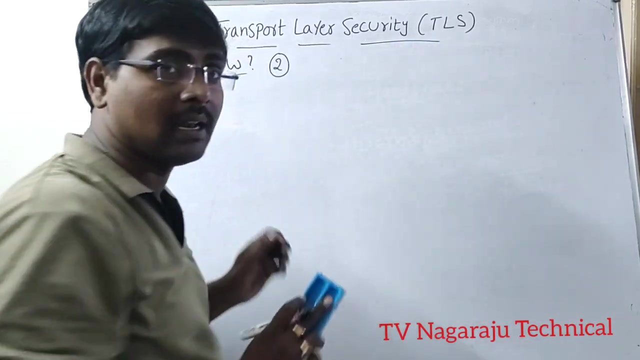 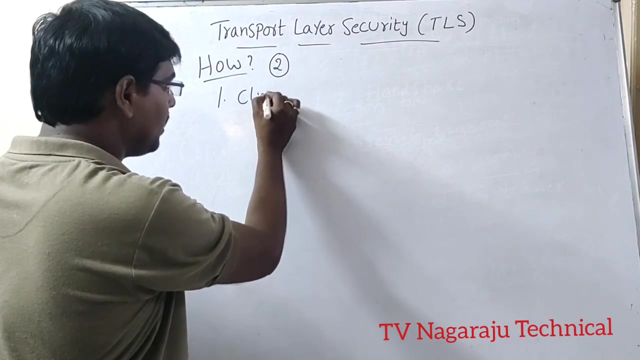 Second one is handshake process. Okay, So almost These are similar to SSL. Here also same TLS record protocol, TLS handshake process. Now I will explain the handshake process of TLS. What is the concept? Very, very simple In the first step: client. 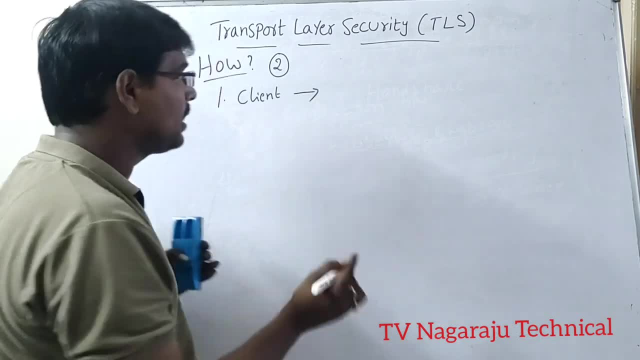 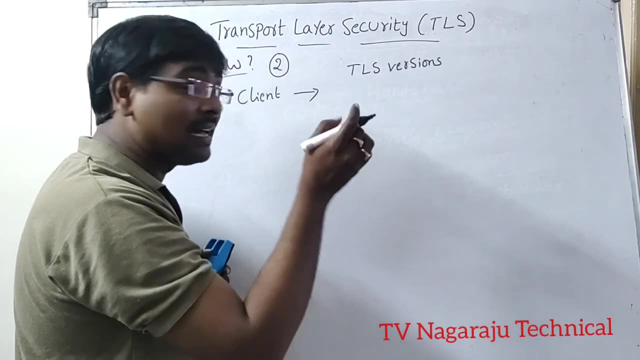 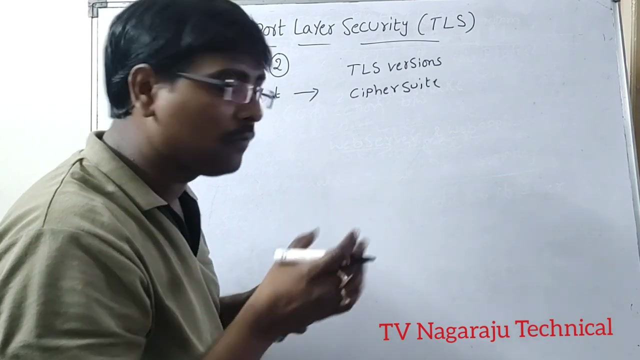 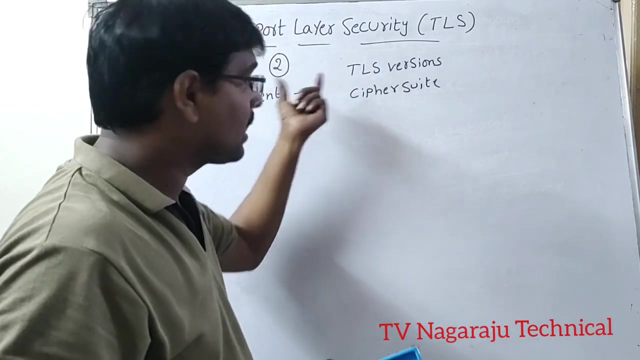 Client send some information to the server. What is the information? Different versions of TLS Along with the suggestions of cipher suite. So just two different versions of TLS along with the suggestions of cipher suite. These two are generated by the client and sent to the server. 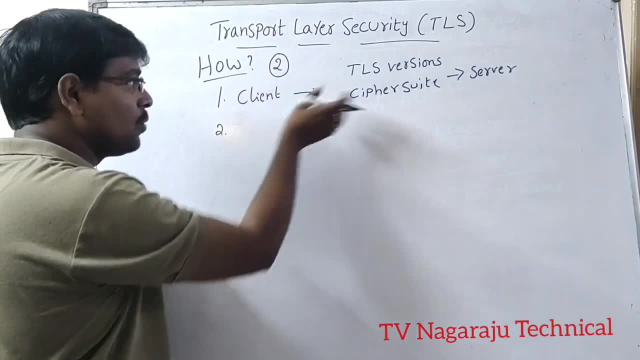 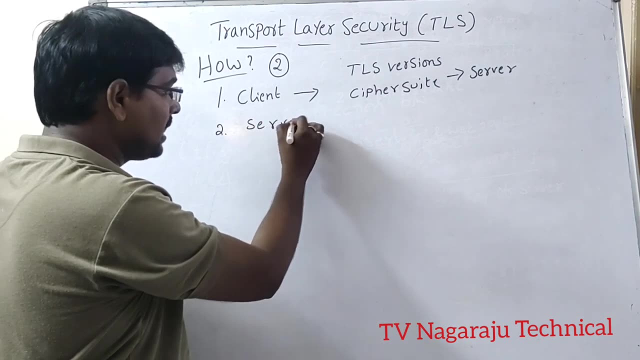 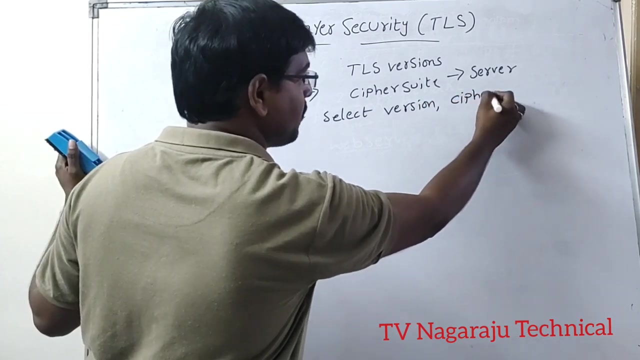 Sent to the server. What happened Once the server receives this information, based on the options of the client server. опрос to DLP. select Cipher Suite For initial 열호 to TLS. select the specific version of TLS and cipher suite. 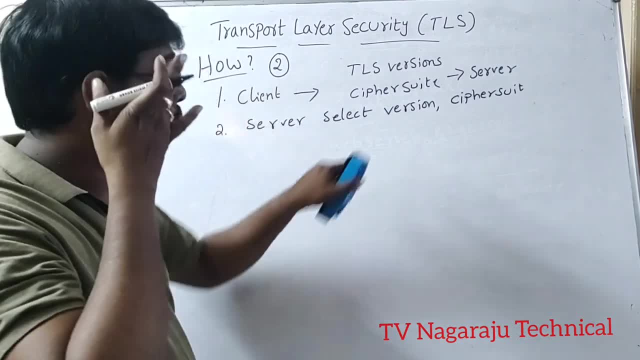 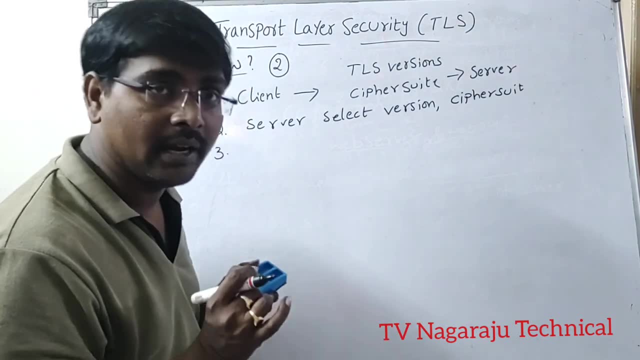 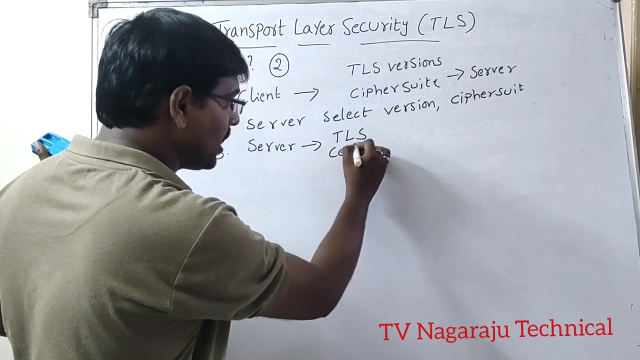 That means initiates the connection Once. accept means it initiates the connection Once the connection is initiatedresult to TLS immediately. server sends TLS certificate. Server sends TLS certificate to the client immediately. Next method: To directly use the connection: Okay. 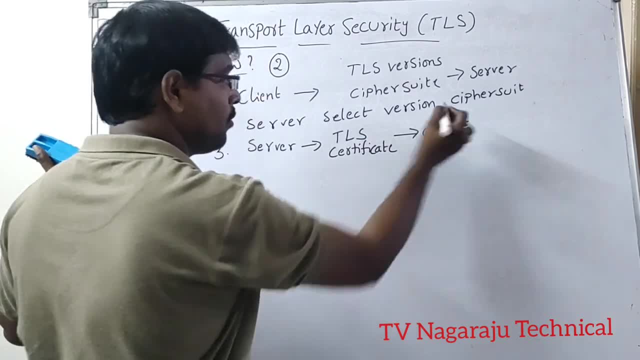 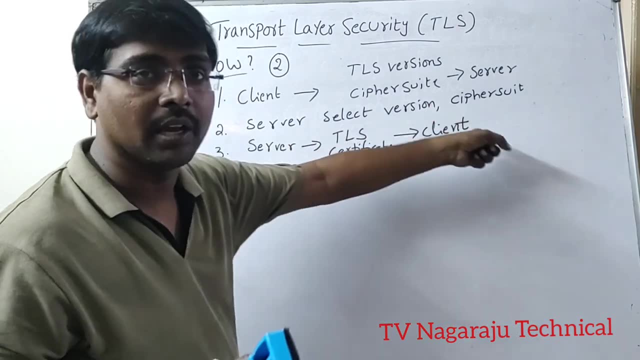 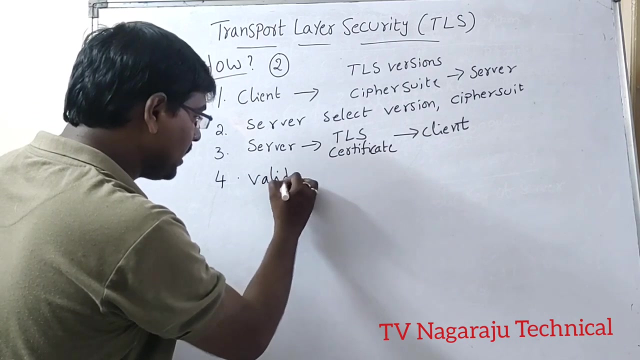 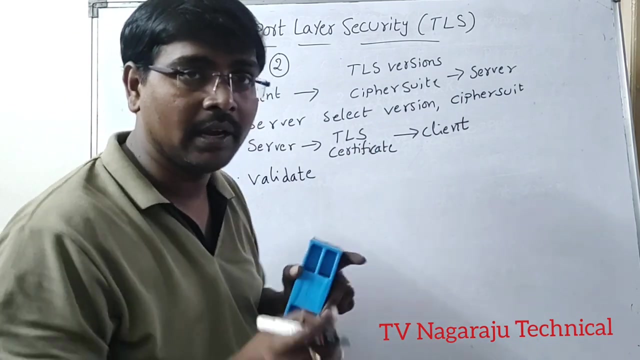 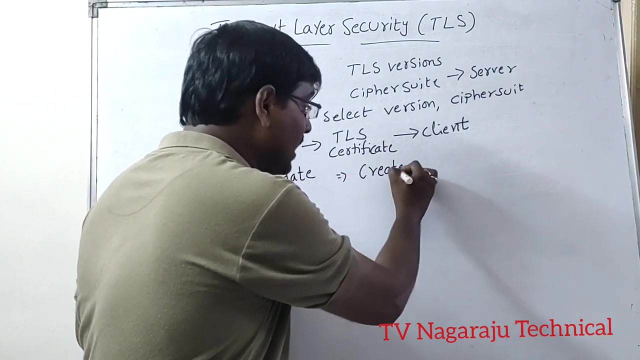 TLS certificate to the client. why? for authentication of server. for authentication of server, he says TLS certificate to the client. once the client receives the TLS certificate of the server, and immediately he validate the server, immediately the client validate the certificate. and if the certificate is valid, if the certificate is valid, now that line to create every. 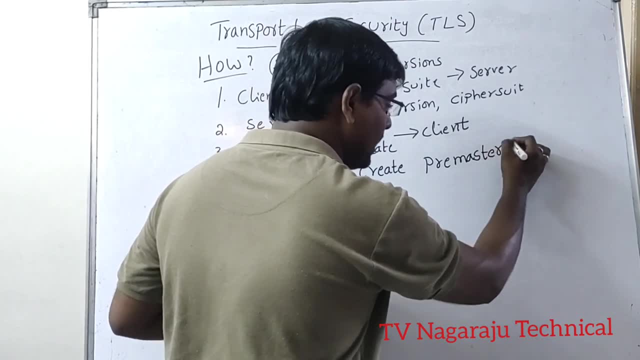 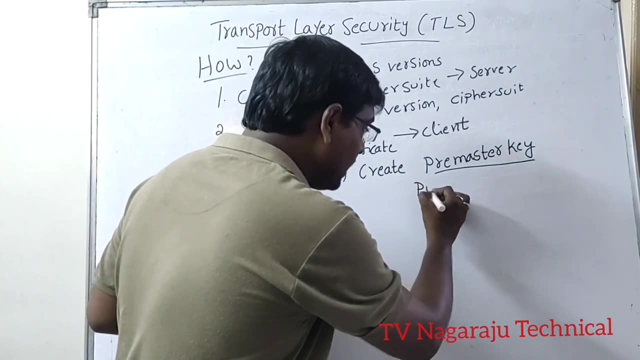 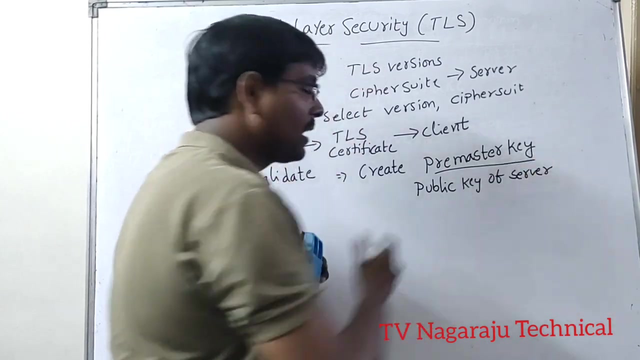 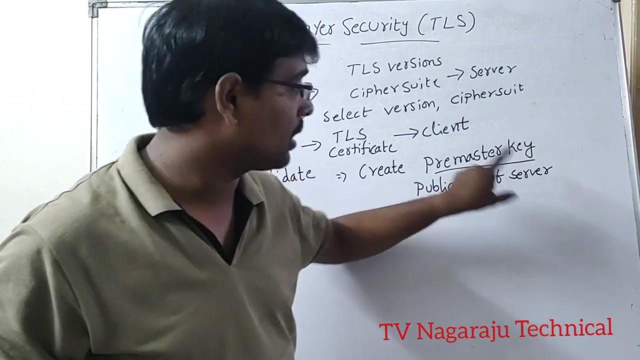 master key that claim to create if remaster key and that master key is encrypted by using public key of server. so that claim to create a pre master key and and that is encrypted by using public key of server. now the question is how the client know public. 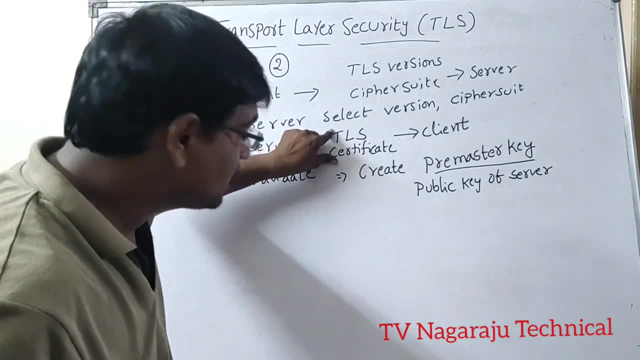 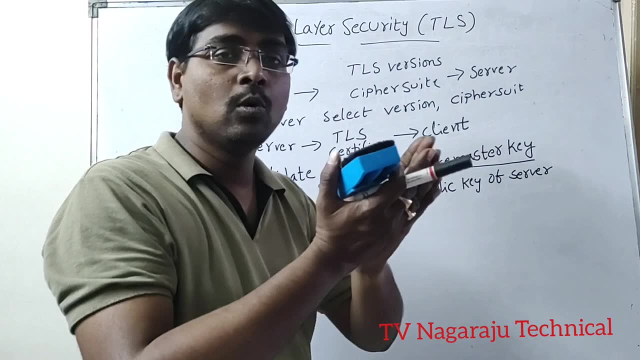 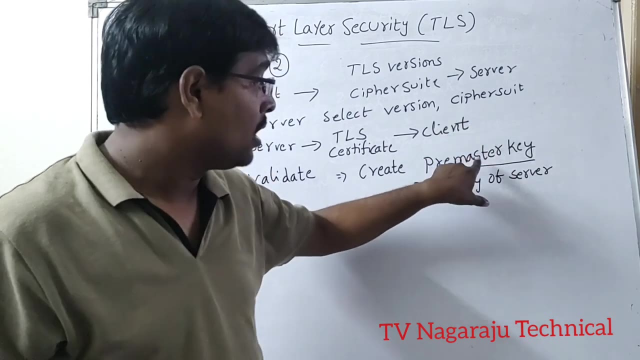 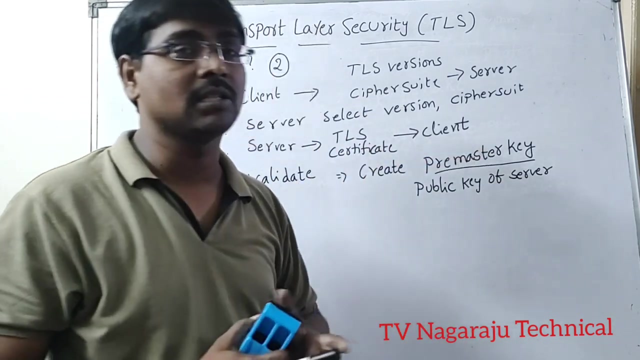 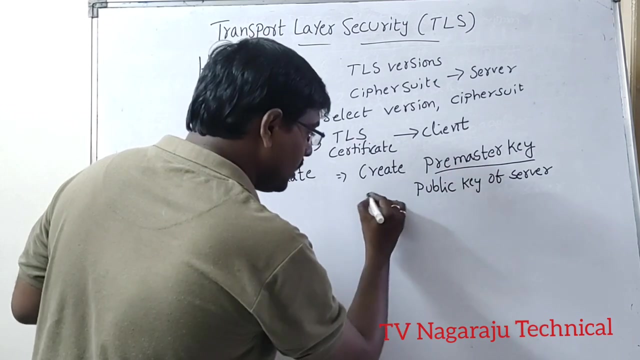 key of server. remember, the certificates itself contains the public key. once that is received by the client, automatically client knows the public key of the server. by using that public key, pre master key is generated. now, who decrypt only the server which consists of private key? then only decrypt the message, then only only that one, only decrypt the message. okay, after creation of this one. 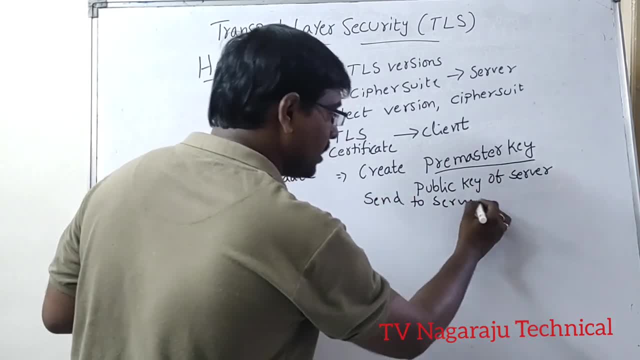 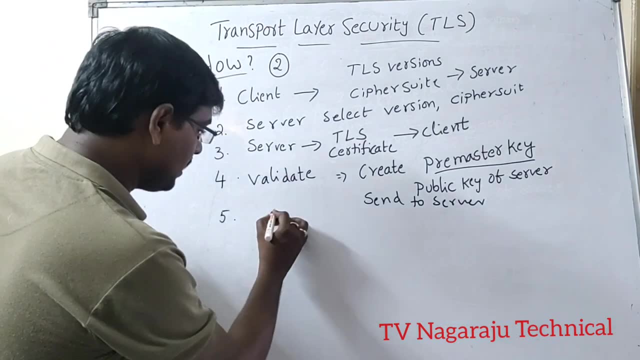 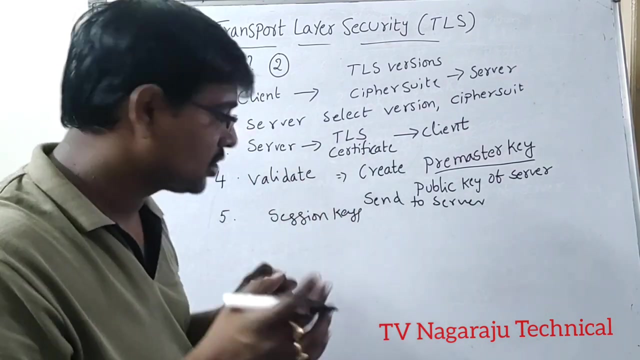 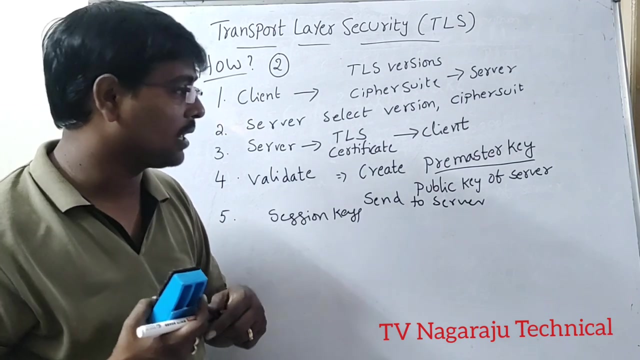 send to the server. after creation, send the pre-master key to the server. now what happened? client and server generate session key keys for transfer the messages to the connection. client and server generate session keys by using symmetric encryption algorithm and based on pre-master key. whatever the master key you are, 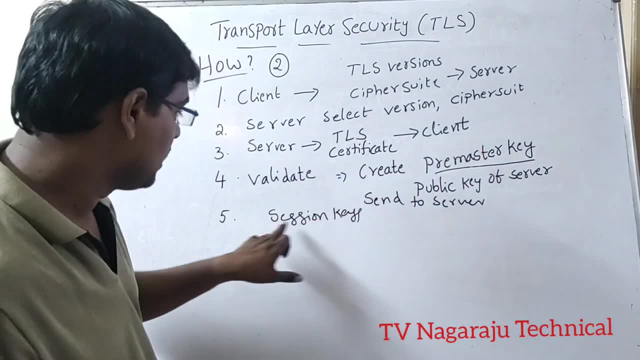 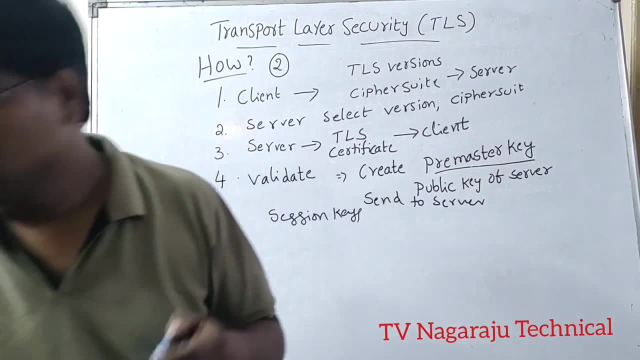 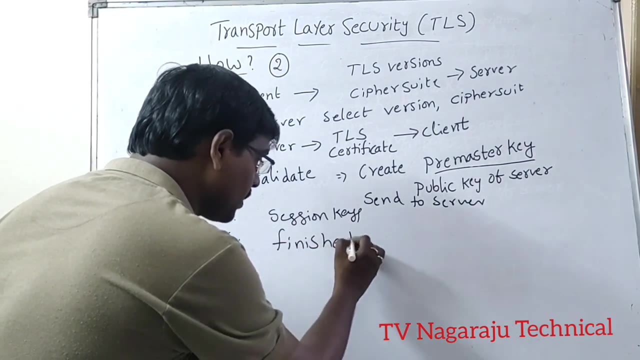 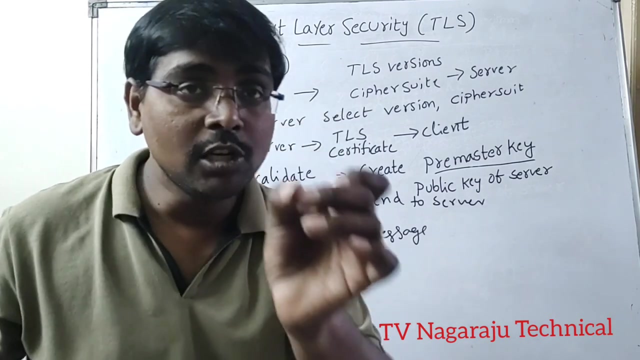 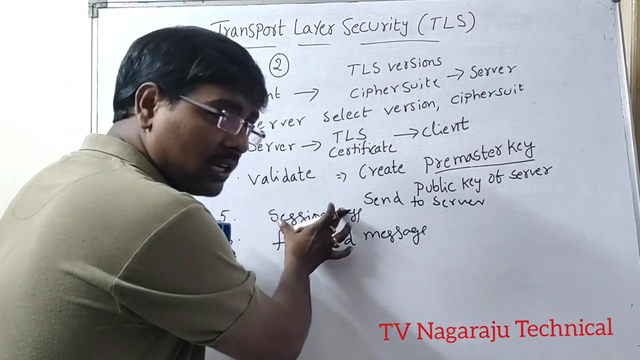 getting. by using this pre-master key, the client and server generates session keys. okay, once the session keys are generated, now both and server have a finished message. both client and server have a finished message. that finished message is encrypted by using session key. i think you got the point. once the session keys are, 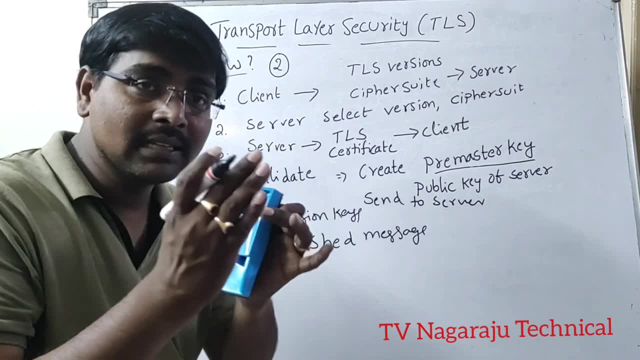 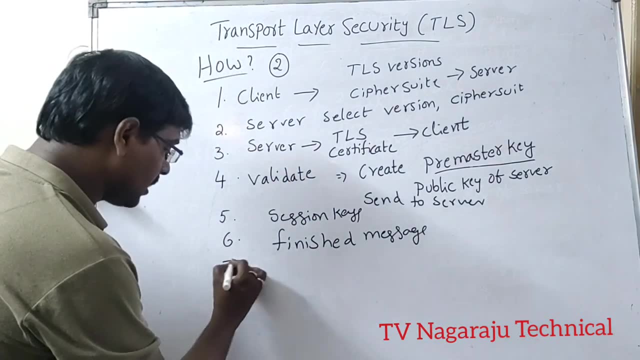 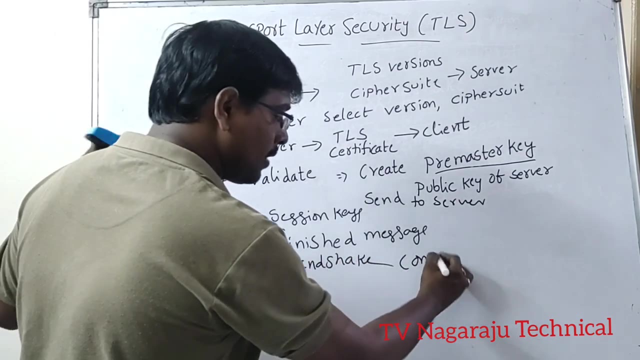 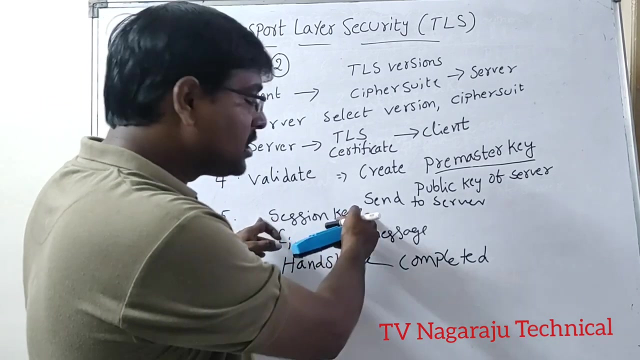 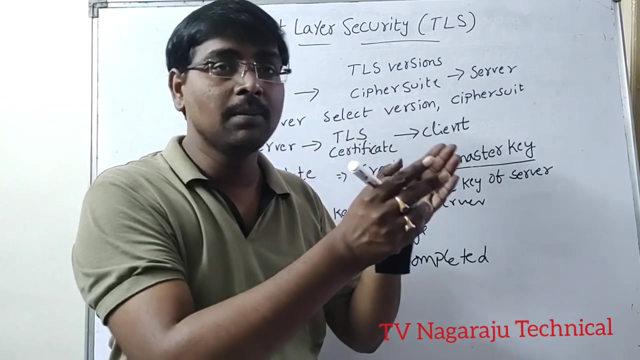 generated. after that one client and server have finished message. that message is encrypted by using session key. finally, the handshake process is completed. finally, the handshake process is completed. okay, and during this process for generation of inuq session key for each and every connection, we are using symmetric encryption algorithm by the first layer tls record protocol. 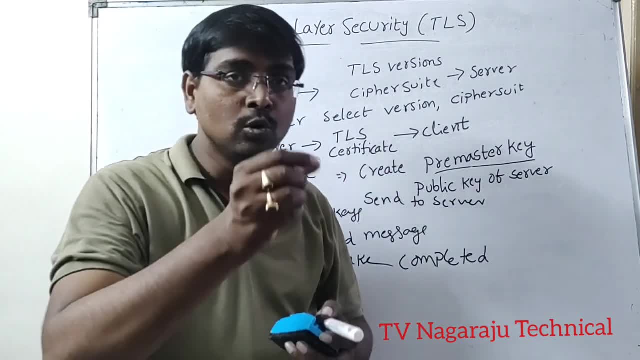 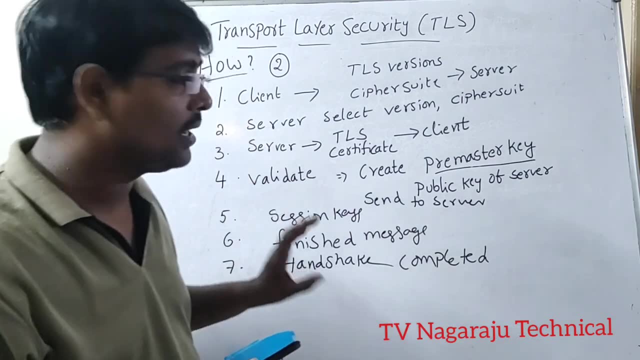 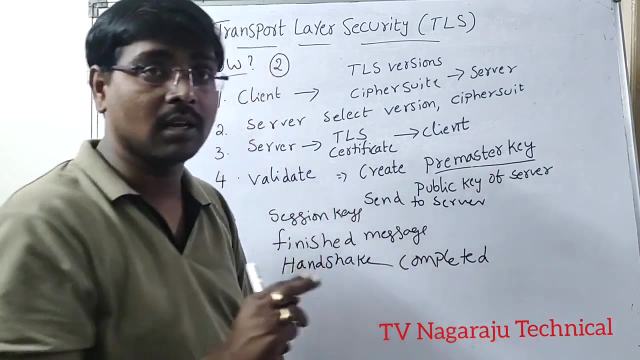 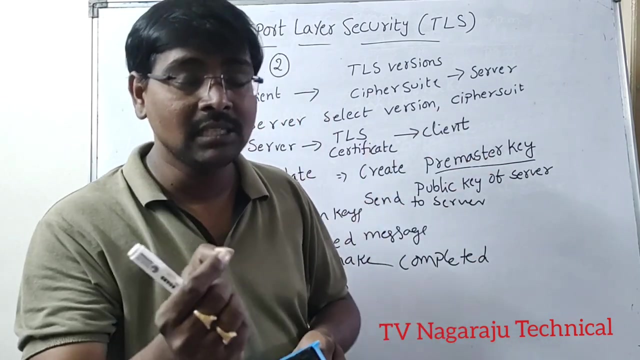 now tls record protocol uses symmetric encryption algorithms for generating session keys. for generating session keys, not only that one, the tls record protocol. first one is generation of session keys. one more thing is there: whatever the message we have for that message, add a message authentication code. but here: 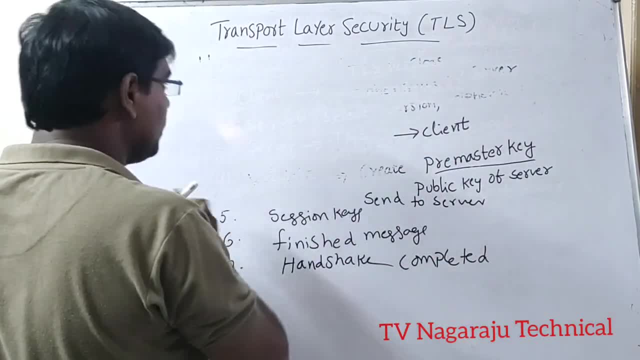 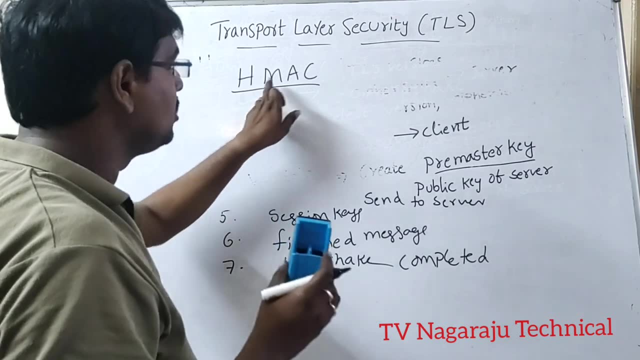 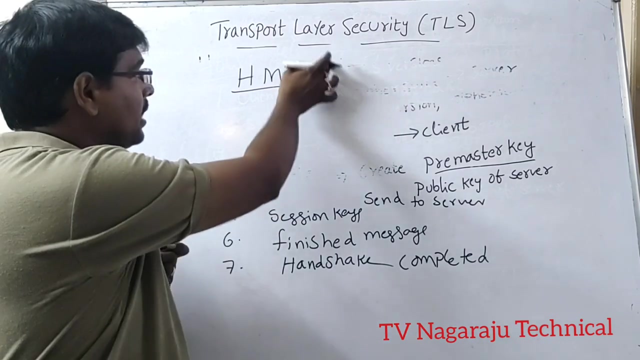 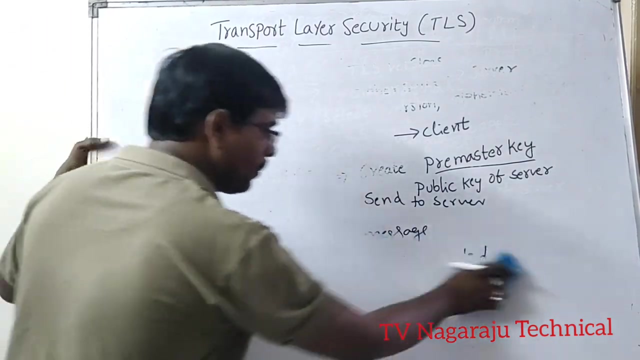 what the message authentication code they are adding. the tls protocol uses hmac hash based message authentication code. this is added to the data. this is added to the data. this is done by tls record protocol. okay, now you understand one point: how the tls certificate validate the client and server. 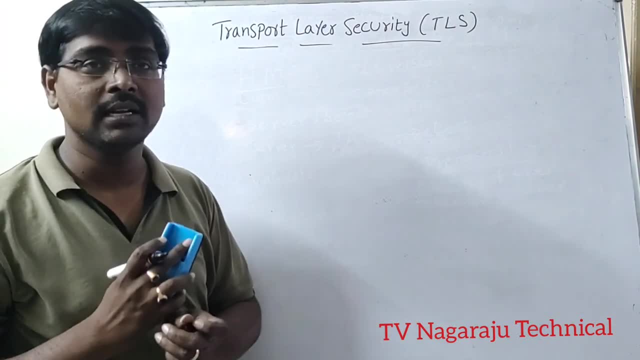 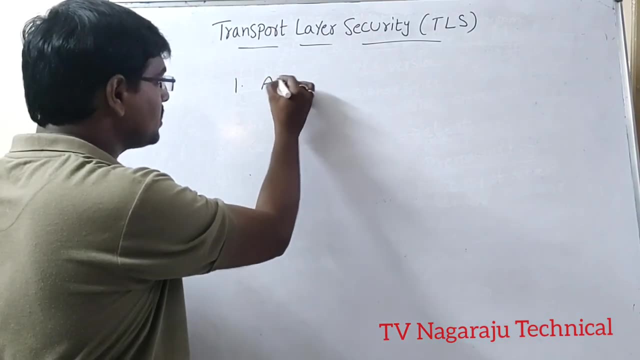 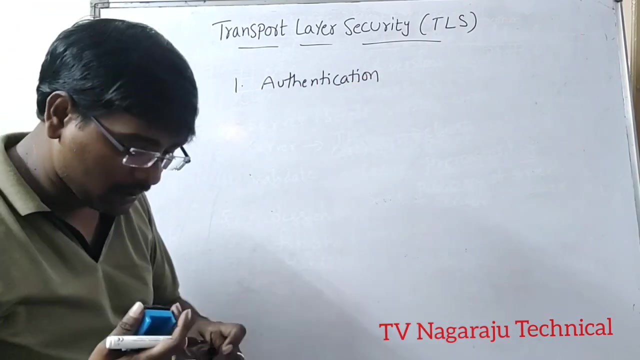 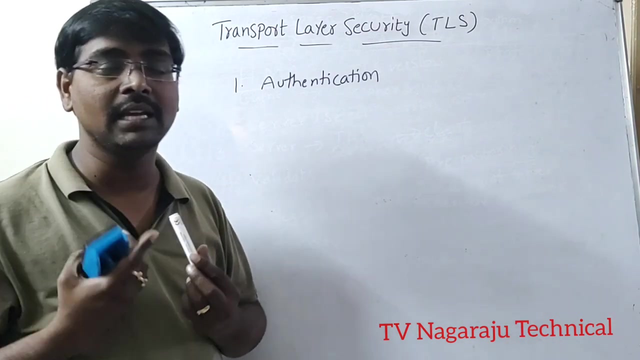 How the message is transformed between client and server. Mainly, TLS provides three services. The main three services are Everywhere: authentication, Yes or no. Authentication means both the parties have to identity Transfer the identities between each other. Then only he is the original author, That is original client. 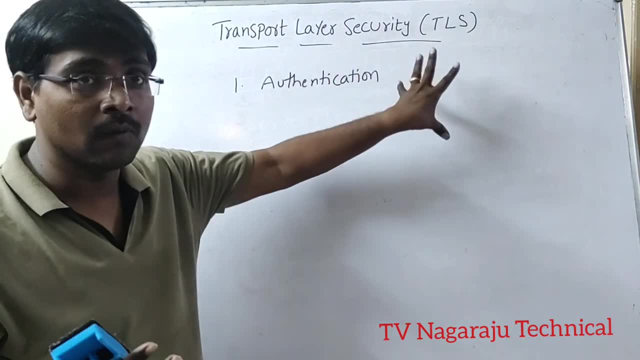 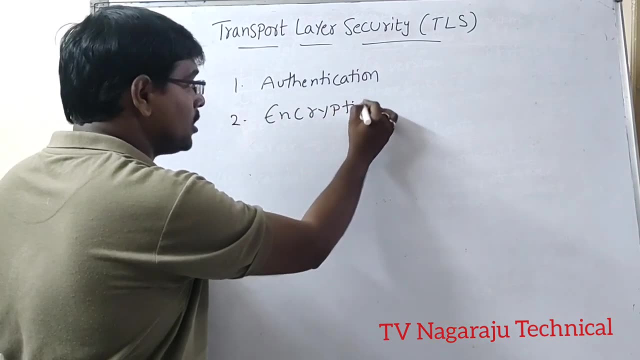 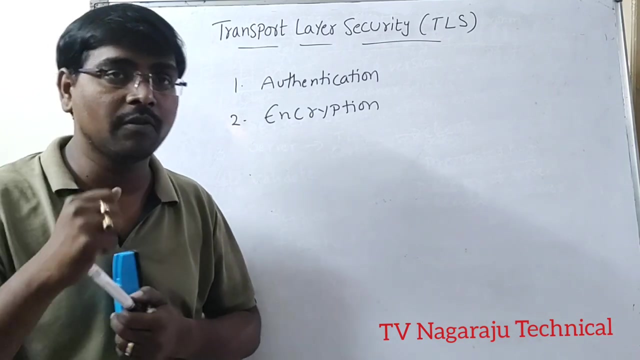 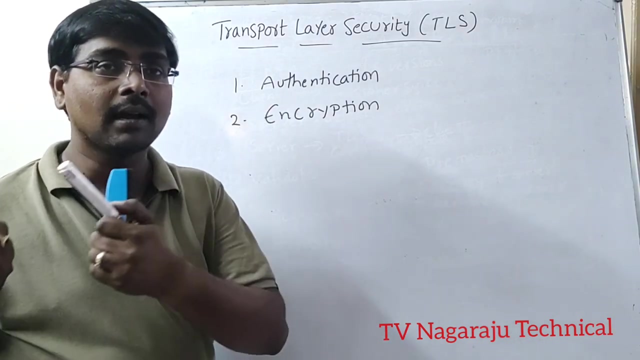 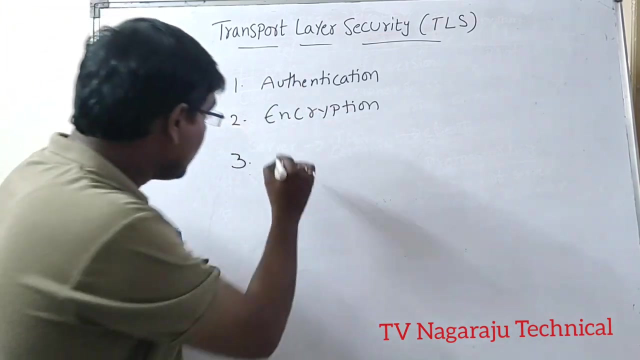 He is the original sender. No other person is involved. Authentication, And next one is encryption. So it uses different symmetric and asymmetric encryption algorithms For exchange of data. Means unauthorized person unable to access Simply hide the data from unauthorized person. Encryption, And after this, authentication And encryption, And the next one is integrity. 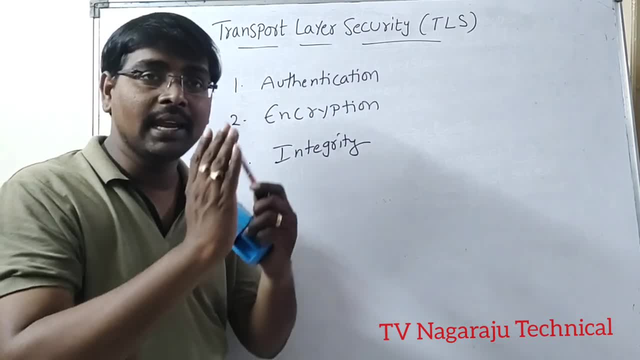 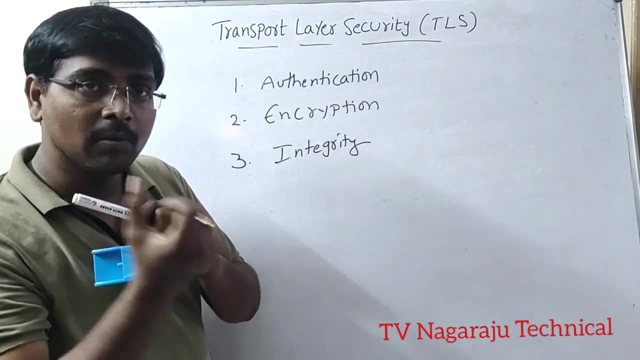 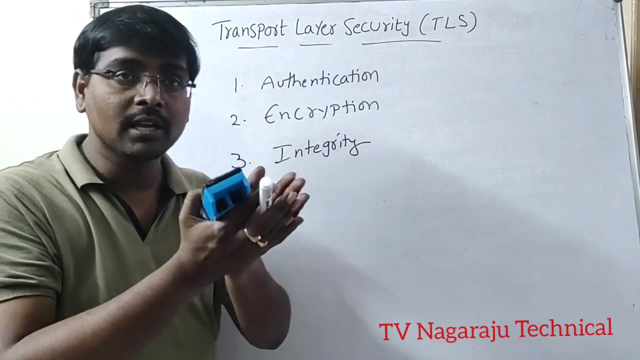 You know the meaning: Integrity. Once the data is transferred During the process, Once the delivered from the sender Before received by the receiver, There is no modification of the data. There is no modification of the data. That means forgery is not happened. How can you say that? 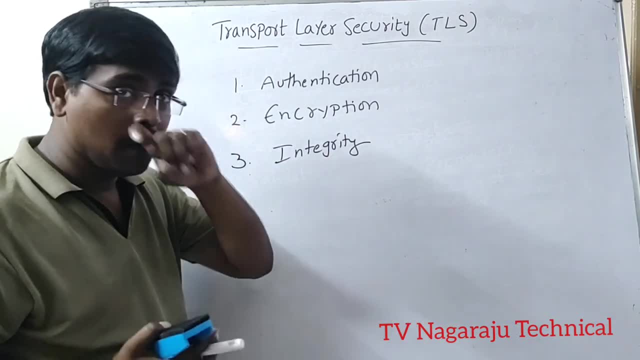 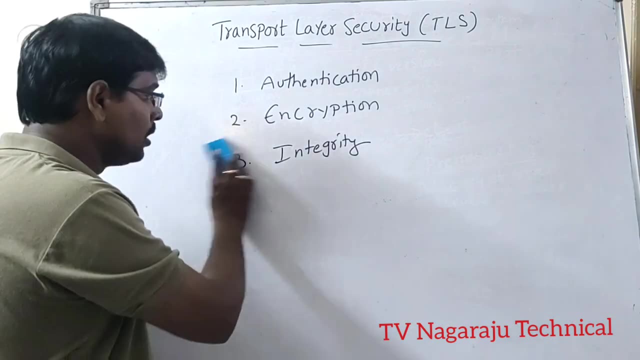 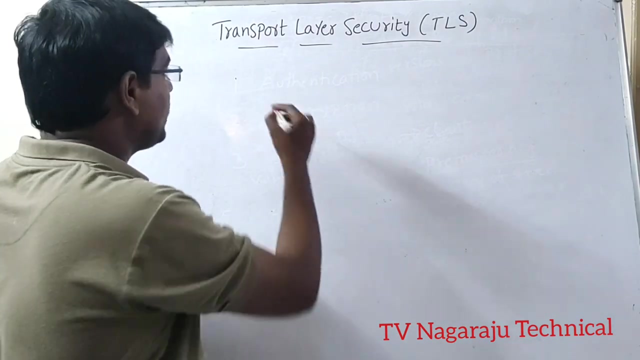 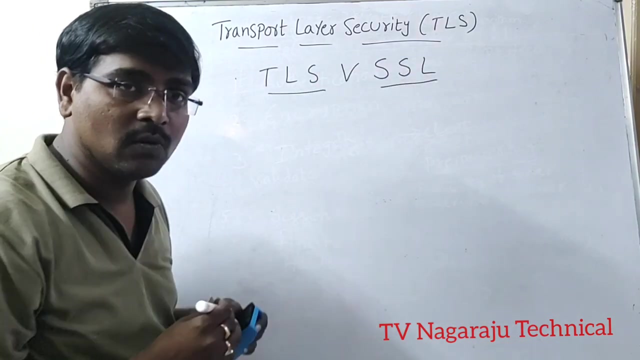 Based on the message authentication Code. Based on message authentication code. These are the main services that are provided by TLS. Now I will give you one very, very important point. The point is: What is the difference between TLS and SSL? So in the last session, we discussed SSL. 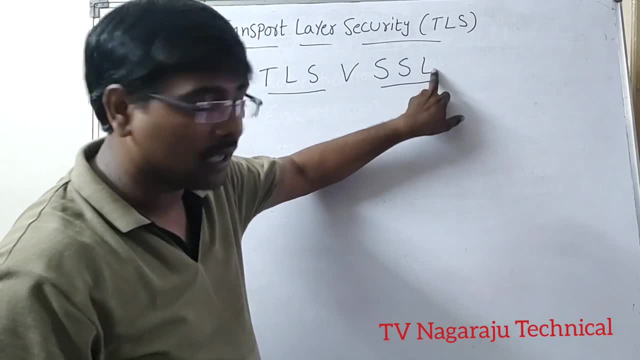 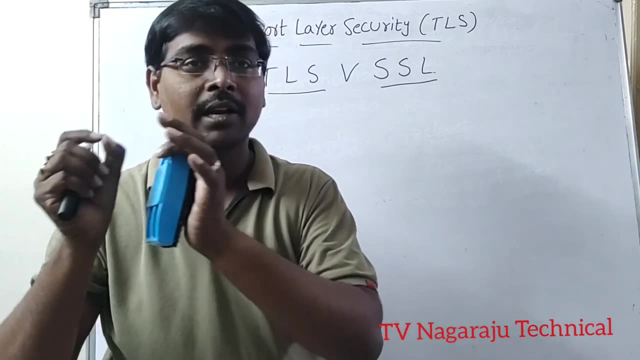 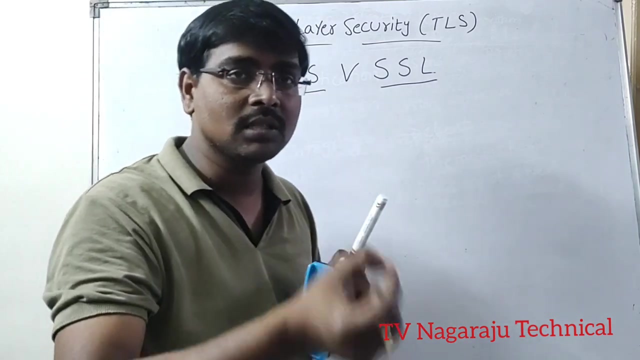 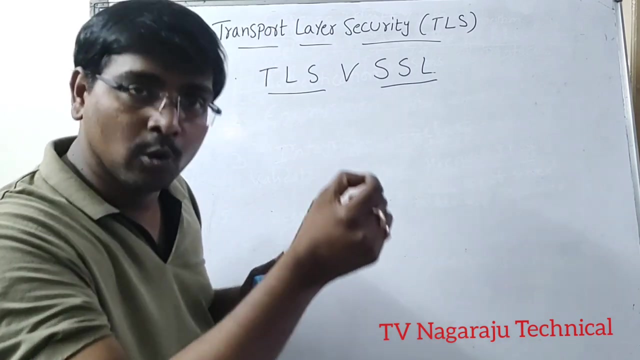 Means secure socket layer, Transport layer, Support layer security. Remember, TLS is not a different topic of SSL. TLS is an initiation In the simple sense. A older version of SSL Simply First to SSL 1.0, 2.0 And SSL 3.0 is completed. 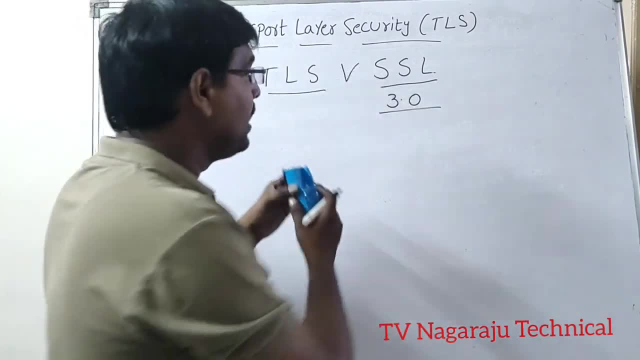 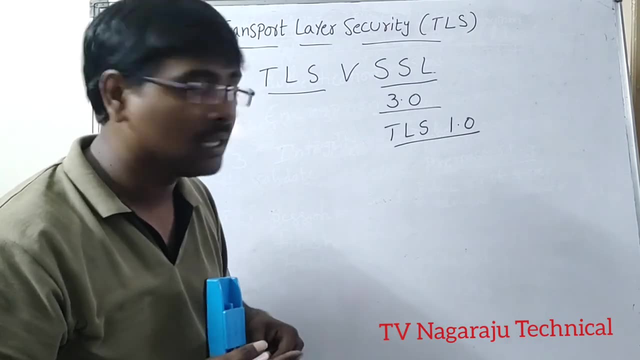 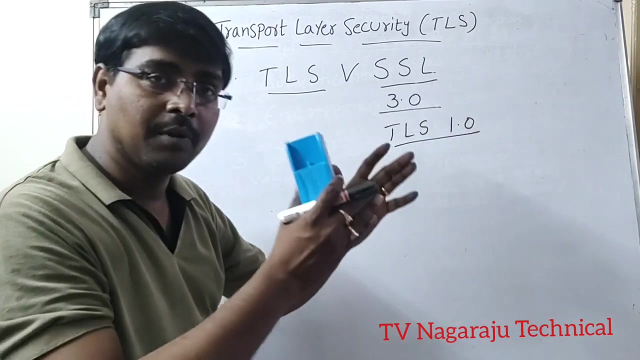 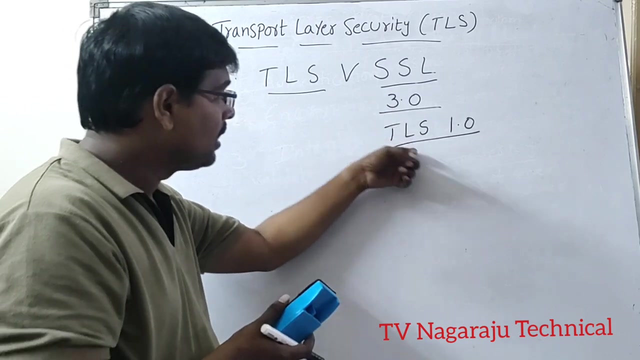 After SSL 3.0, Immediately They are developing TLS 1.0. That means TLS is generated from the older version of SSL. Everything is same, Whatever the security that provided by SSL. TLS also do the same thing. Why It is the next version? The only thing is the organizations are changed. 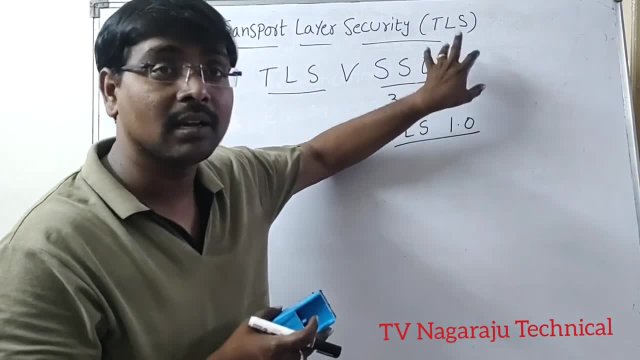 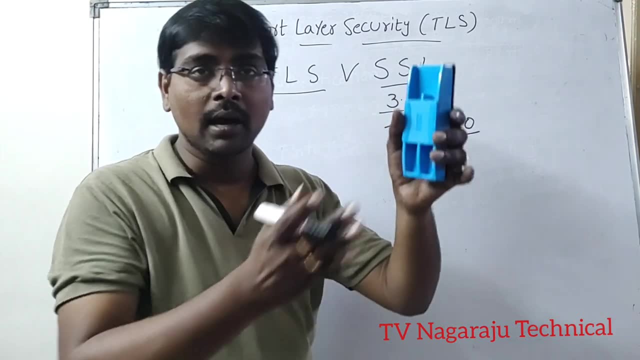 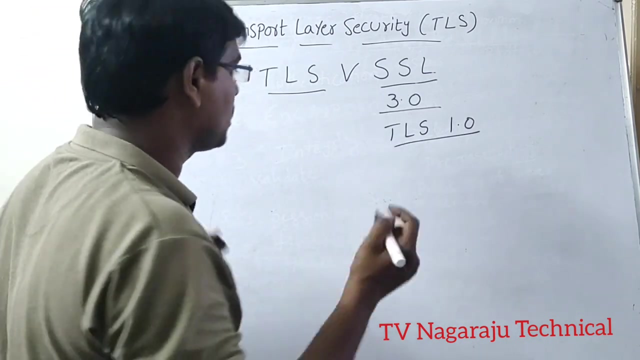 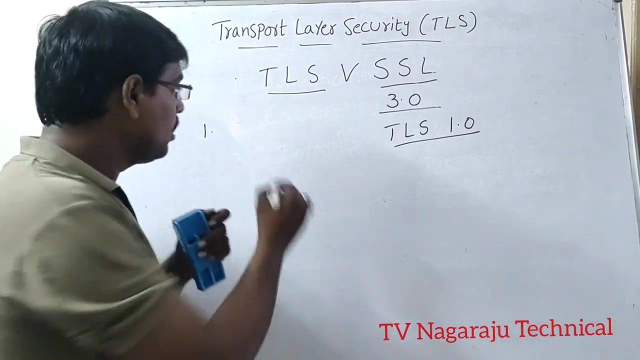 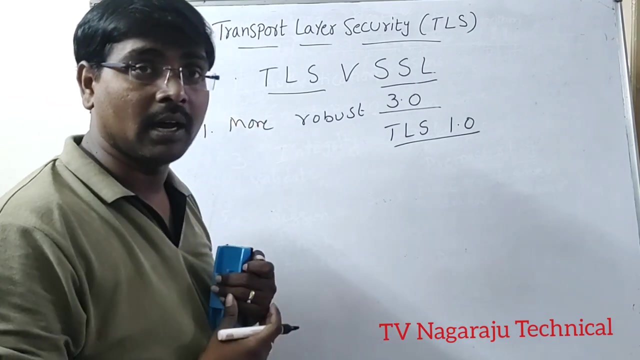 For example, SSL is provided by Netscape And TLS is provided by Internet Engineering Task Force, So organizations vary. That is the reason. just to change the name And some minute. small differences are there. TLS uses more robust authentication process, More More Robust authentication process And more robust encryption algorithms. 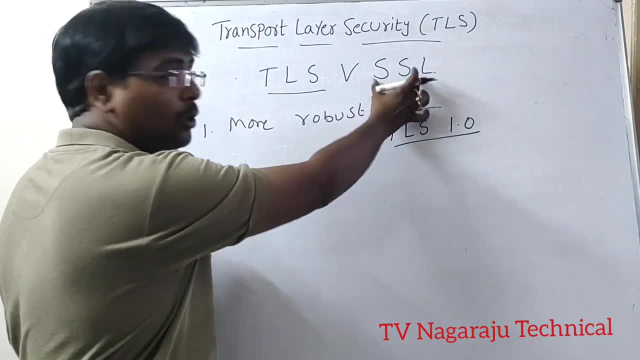 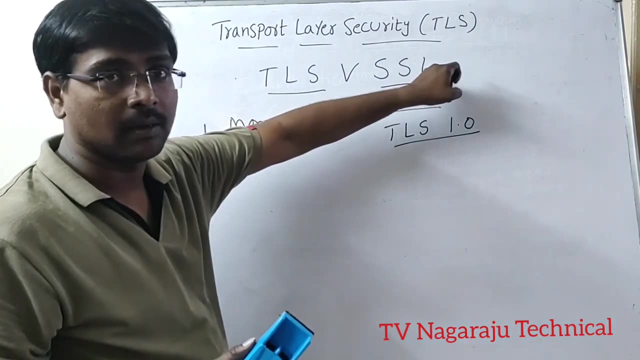 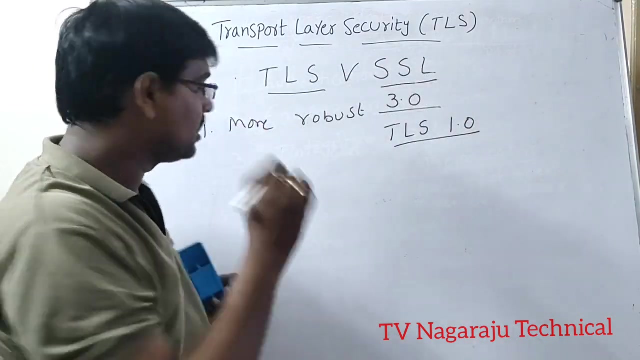 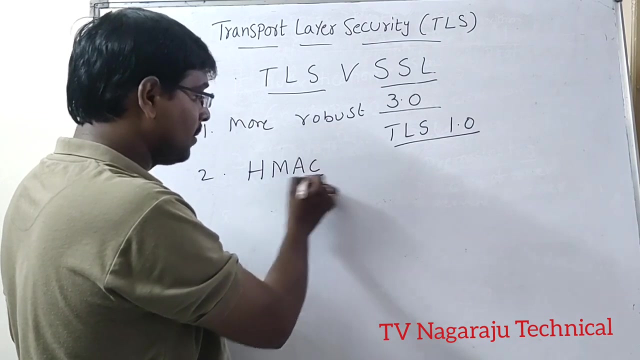 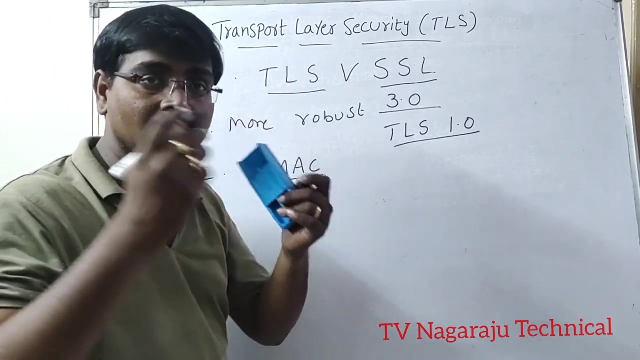 More robust encryption algorithms. Compare it to SSL. That is the reason TLS provides more security than SSL. That means TLS certificate has more value than SSL certificate. That is one reason. Another one is TLS uses HMAC algorithm: Hash based message authentication code. Once they encrypted, We are adding the message authentication code to achieve the integrity.